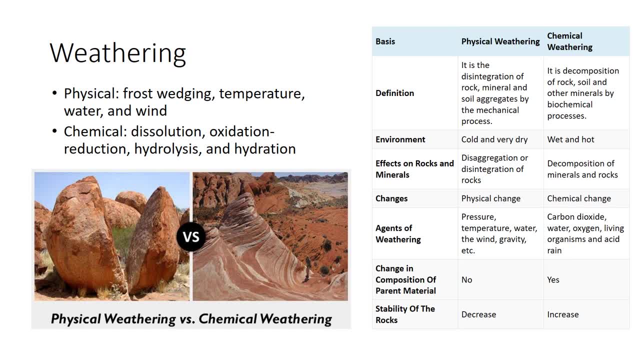 frost. wedging occurs when water freezes and expands in rocks or cracks in that rock, causing it to break apart. The alternate expansion and contraction of rock caused by heating and cooling cycles also stresses the fabric of rock, cause rock to fracture or outer layers to peel away. Rain, running water and windblown 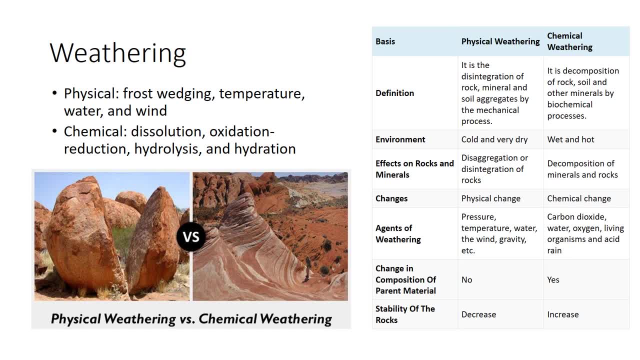 dust also wear away at rock surfaces. Chemical weathering changes the chemical makeup of rock and breaks it down. A common process is dissolution Minerals dissolving in water. In hydrolysis, minerals react with the hydrogen that is in the water molecule, splitting the water apart. For example, the feldspar mineral. 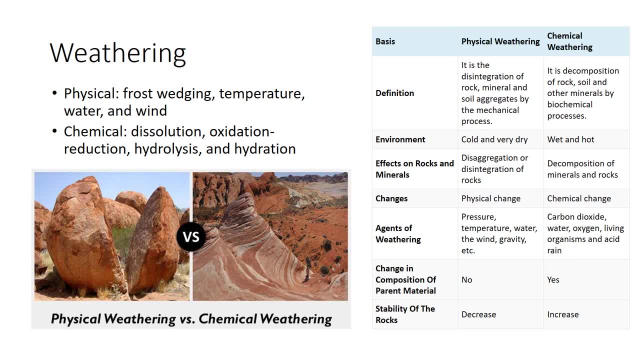 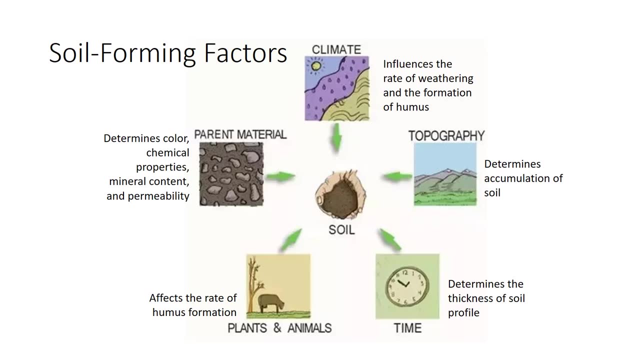 orthoclase undergoes hydrolysis by replacing the sodium in the mineral with hydrogen, creating a new, softer feldspar. Other processes include hydration, where the water molecule joins the crystalline structure of the mineral, and oxidation reduction. Soil formation does not stop when a layer of young soil covers the surface. The new 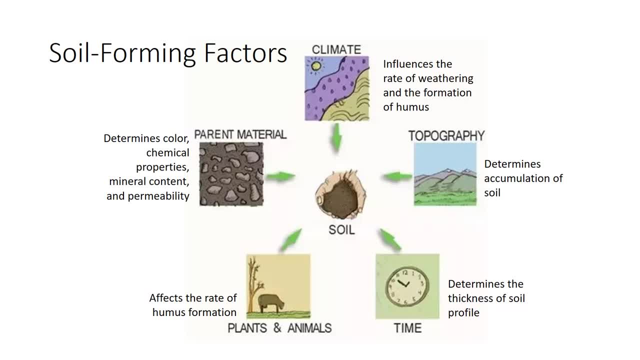 soil continues to age slowly and develops over thousands of years. Soil scientists state that five factors operate during the process of soil genesis and development: Parent material, Climate, Life, Topography, Time. One could say that over time, climate and living things act on parent material with 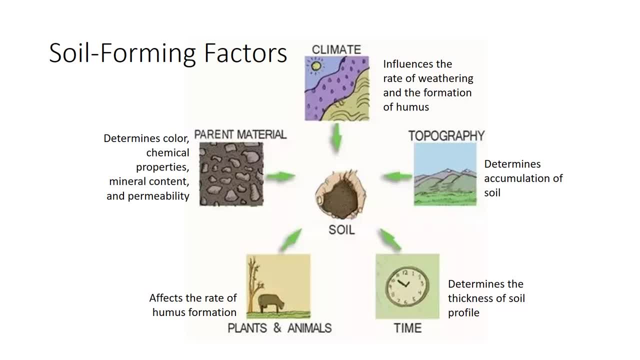 a certain topography to create soil. Some have suggested that human activities might be named a sixth factor. Soil formation begins with rock, which supplies the parent materials for most soils. Before studying the five factors, let us take a look at Rock Formation. Rock Formation is the process in which rock 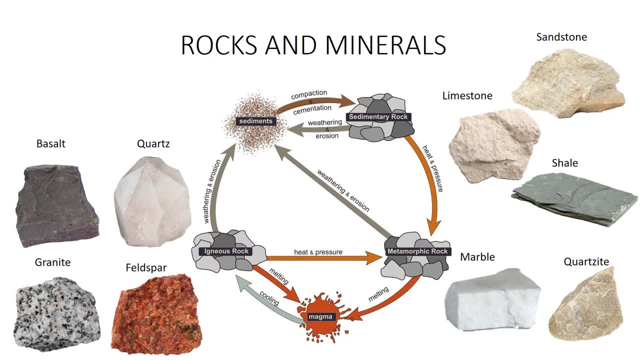 of Earth's crust. The original source of most soils is rock, the solid, unweathered material of the Earth's crust. Solid rock breaks into smaller particles, which are the parent materials of soil. Rock is a mixture of minerals that, when broken down, supply. 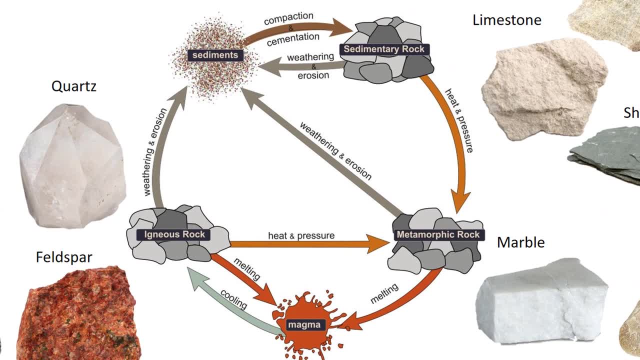 plant nutrients. Geologists classify rock into three broad types: igneous, sedimentary and metamorphic. Igneous rock, created by the cooling and solidification of molten materials from deep in the Earth, contains minerals that supply 13 of the 17 plant nutrients. 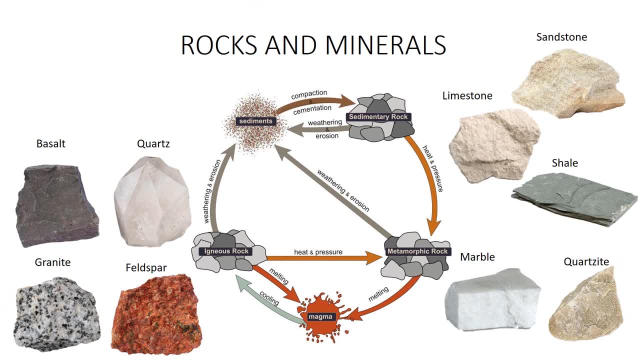 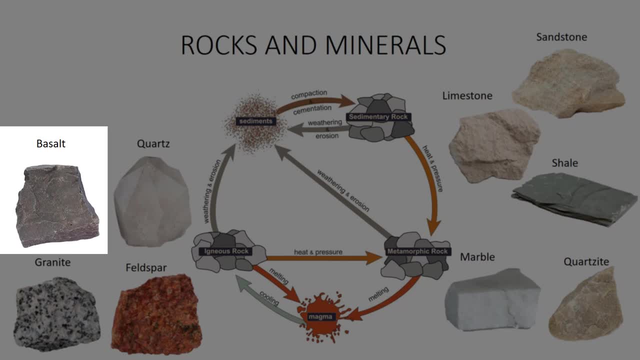 Igneous rock may be coarse-grained, with grains and crystals large enough to see with the eye. Basalt is fine-grained, Darker-colored igneous rocks tend to weather more easily and contain more iron and calcium. Granite is a hard, coarse-grained rock made of feldspar. 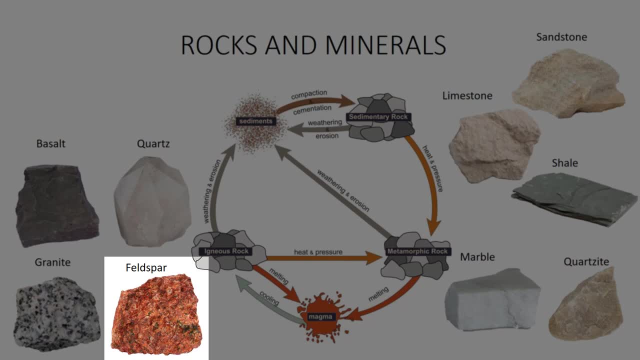 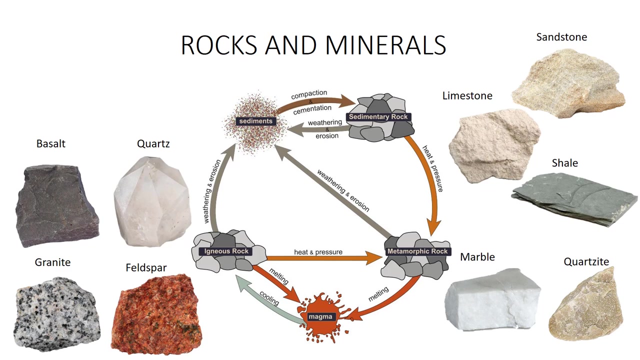 quartz and other minerals. Feldspar, a fairly soft mineral containing potassium and calcium, weathers easily to clay. Quartz, a very hard and resistant mineral, weathers slowly to sand. Most of the crust is igneous rock, but it is only one-quarter of the Earth's surface. 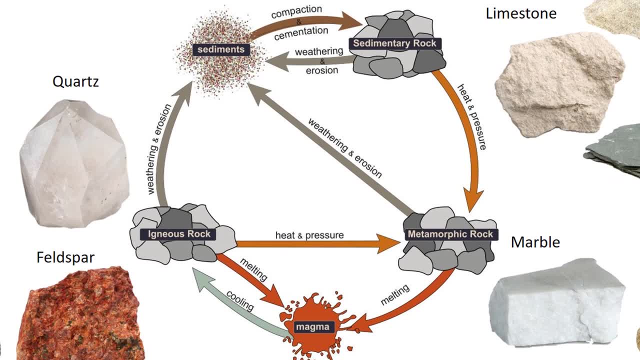 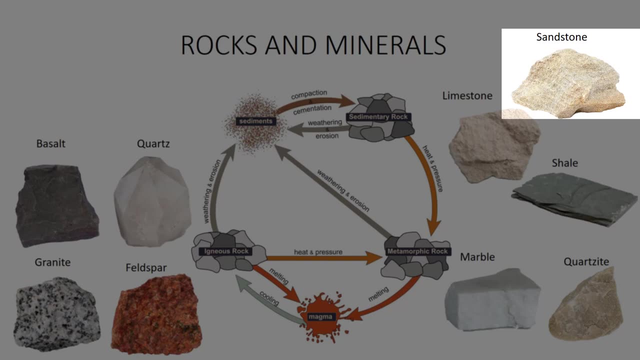 Sedimentary rock overlays three-quarters of the igneous rock. Sedimentary rock forms when loose materials such as mud or sand are deposited by water, wind or other agents, slowly cemented by chemicals or pressure into rock. Sand deposits can solidify to sandstone. a 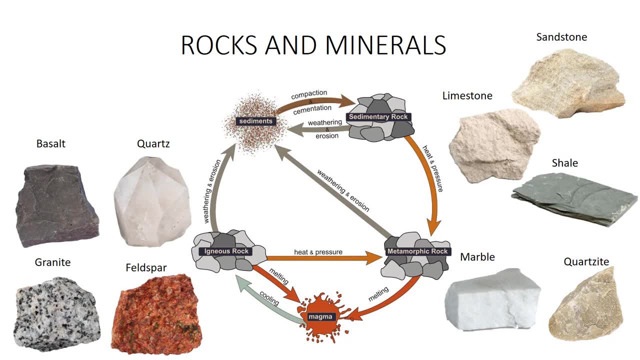 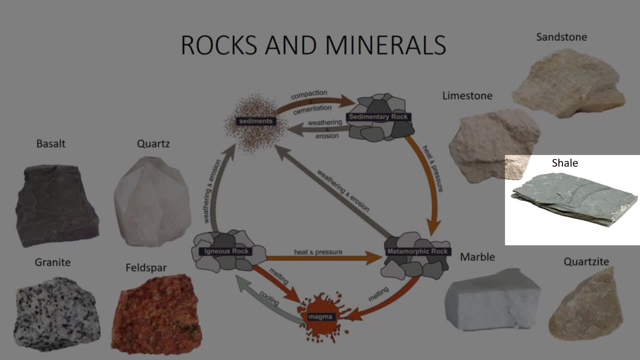 light-colored, coarsely-grained rock. Loosely cemented sandstone weathers easily to release sand. Mud deposits form shale. a fine-grained rock Limestone forms when calcium-rich grains of calcite settle out of ocean water. 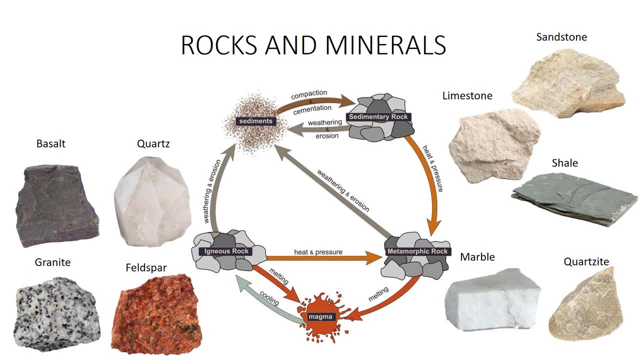 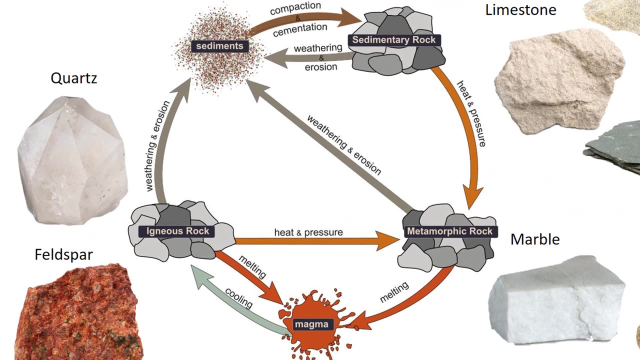 Many American soils are derived from sandstone and limestone. These soils are generally infertile and dry. Limestone is high in calcium and weathers easily to soils high in pH, calcium and magnesium. Metamorphic rock forms when igneous and sedimentary rocks are subjected to great heat and pressure. 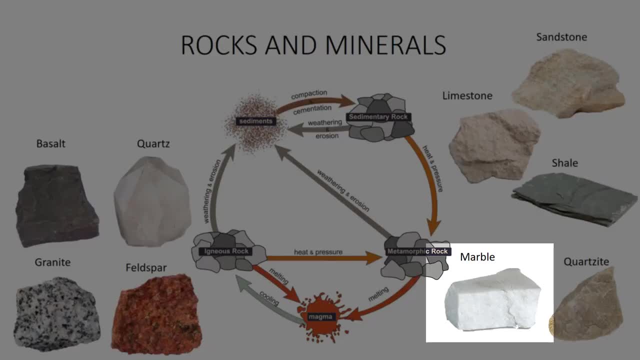 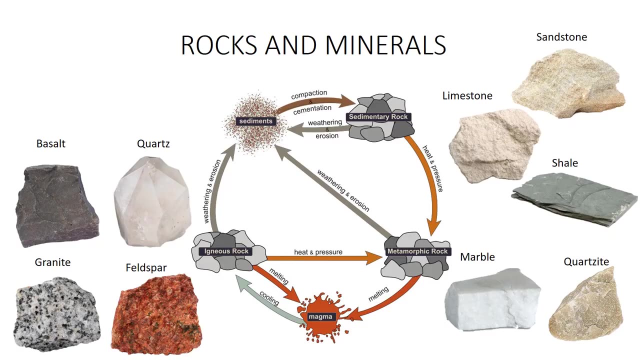 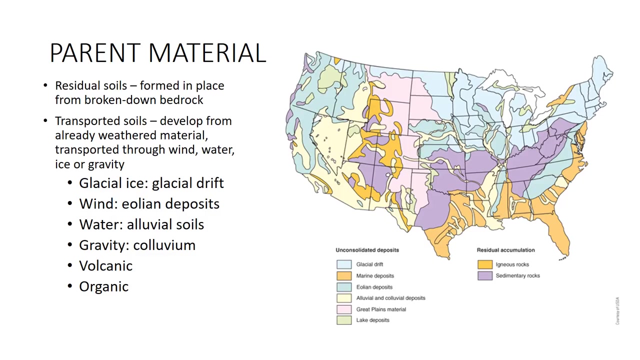 Limestone, which is fairly soft and gritty. changes to marble when subjected to heat and pressure. Sandstone changes to quartzite. Soils from metamorphic rock tend to look like the original sedimentary or igneous rock. Soil genesis is the process of creating soil from parent material. The description of soil. 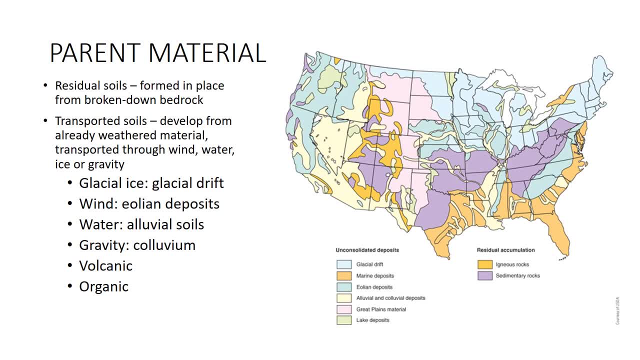 origin earlier in the chapter was a soil formed directly from bedrock. Such a soil might form from the rocks in the rock cycle. These residual soils formed and placed from the residuum of broken-down bedrock are actually less common than soils of parent materials carried from. 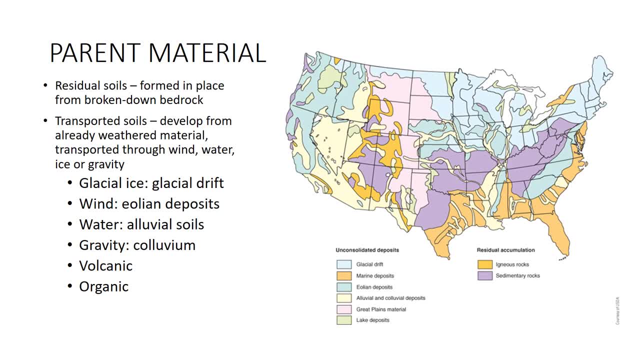 elsewhere by such pervasive agents of transport as wind, water, ice or gravity. Residual soils form slowly. A solid rock must be weathered first. Transported soils develop from already-weathered material, so they develop more quickly. This figure shows parent materials of soils in the United. 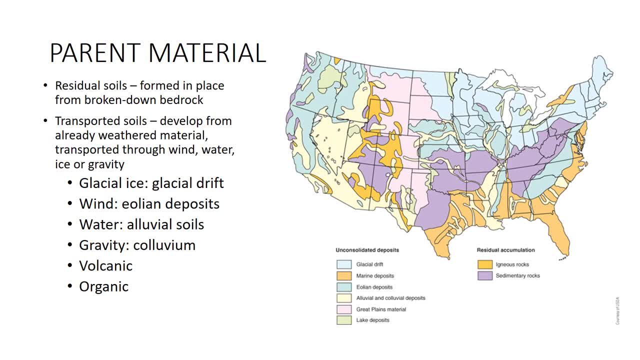 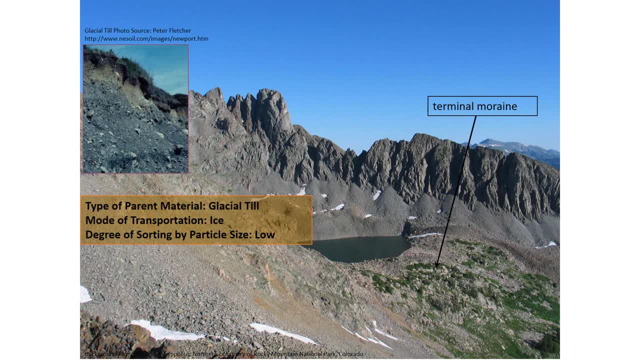 States. Let us look at the agents of transport and the sorts of parent materials they carried. Parent material transported by ice is called glacial till. This parent material is found where glaciers have deposited sedimentary rock. This material is found where glaciers do so with positive material, such as in terminal and lateral moraines. Ice is a pore sort. 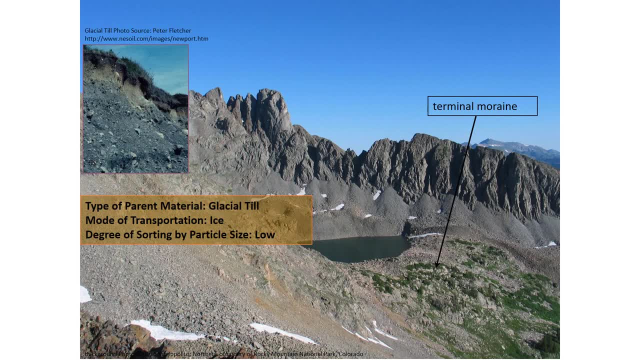 of particles, and thus glacial till Vladimir olevschevich, contained everything from the smallest clayside fraction to rocks, petals and boulders. Glacier is left behind by a distinctive landscape over much of the northern United States and Canada, often rich in wetlands. 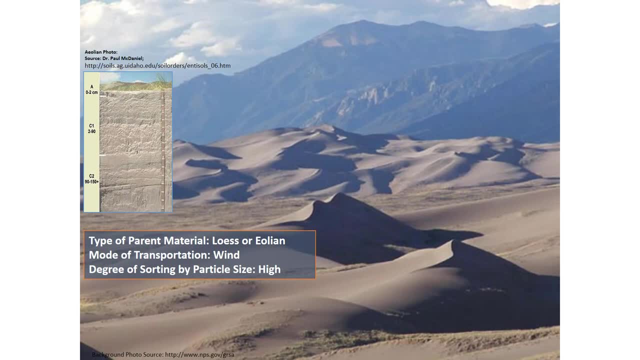 lakes and ponds. Parent material transported by wind is called lois or Aeolian. Wind is a good source of sediment. slimy clay or dew wouldn t shoulders in addition to instability. order of particles: Larger particles tend to bounce on the Earth's surface, while smaller 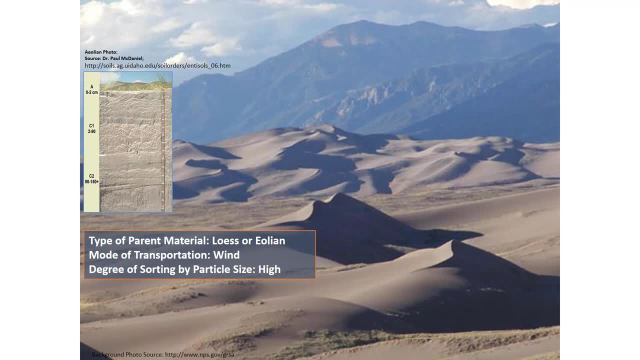 particles are transported greater distances. Loess soils are important agricultural soils in much of Iowa, Illinois and neighboring states. Dust blown from the Sahara Desert of Africa makes a significant contribution to soils of the Caribbean islands, as well as Central and South America Parent material transported by flowing water. 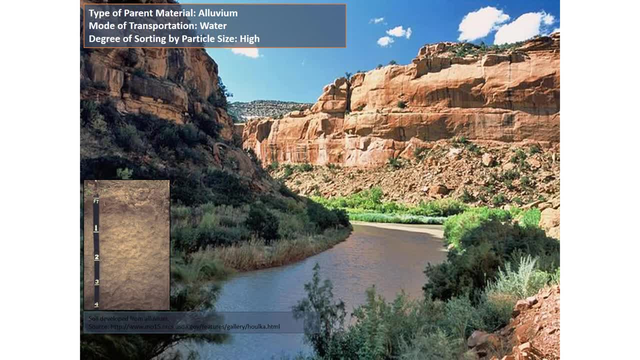 is called alluvium. Water is a good sorter of soil particles. Larger particles settle out of the water first, making levees or floodplains, and smaller particles settle out of the water last, making deltas. Thus you tend to find sand-sized particles closer to the water source and clay-sized particles further away. 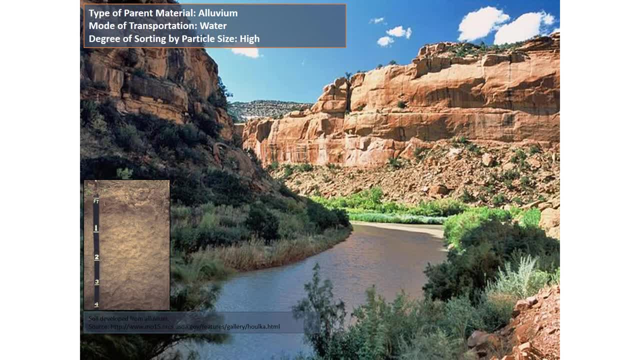 Floodplain soils are especially important along the Mississippi and its tributaries and along rivers that flow into the ocean on the east and gulf coasts. Many important soils of California are from river alluvium. The term lacustrine classifies parent material. 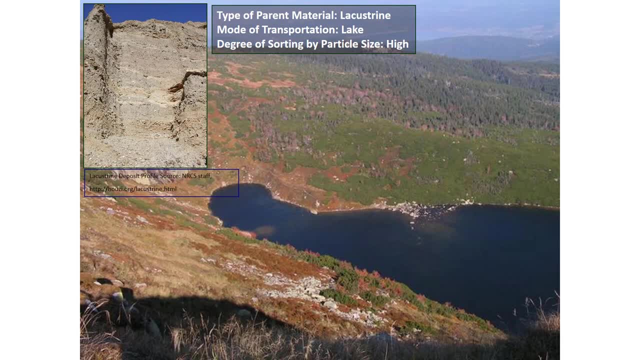 transported by a lake. Water is acting on the parent material, and thus there is a high degree of particle sorting. Most of our lacustrine soils remain from giant glacial lakes that have since dried up, including Glacial Lake, Agassiz of northern California and the Salta. Valley of California. Our most important soils in California have been from a river from late 19th century to the end of the 1960s. Loess is a growing mineral and that's what we need. We have all the resources we need If you know where to get your loess, please. 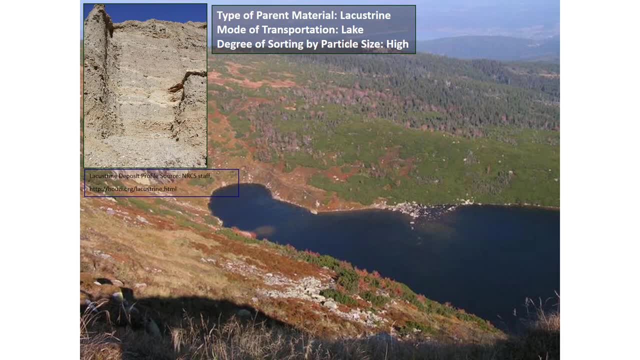 Minnesota, North Dakota and Canada. in Glacial Lake, Bonneville of Utah, When glacial runoff water ran into the lake, the heaviest materials were left near the shore, while the smallest particles were carried to the center of the lake. Lacustrine soils have flat terrain and 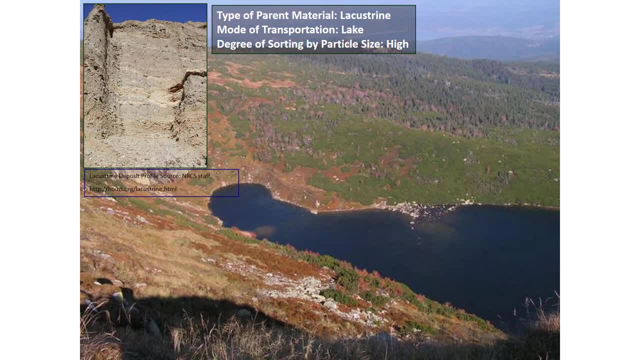 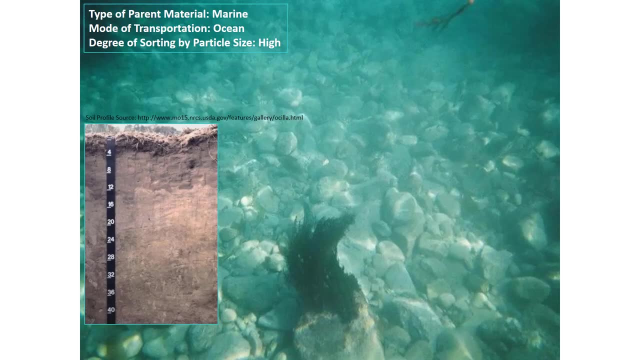 being poorly drained can host rich agriculture with proper artificial drainage but challenge the home and septic field builder. The term marine classifies parent material transported by oceans. Water is acting on the parent material and thus there is a high degree of particle sorting Many scattered soils of the Great Plains and the Imperial. 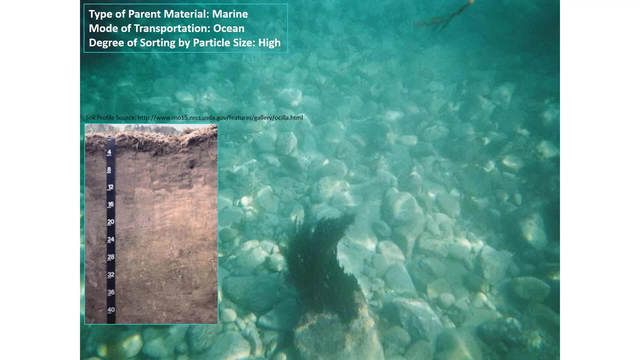 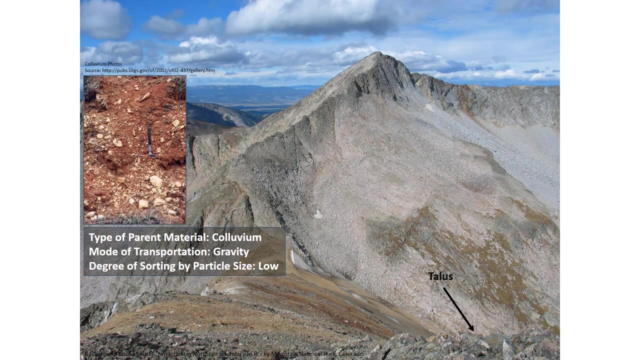 Valley of California are beaches of prehistoric seas that once covered the United States. Other beach soils are common along the Atlantic coastline and the Gulf of Mexico. All these tend to be sandy soils. Sounds like Florida right. The term colluvium classifies parent material. 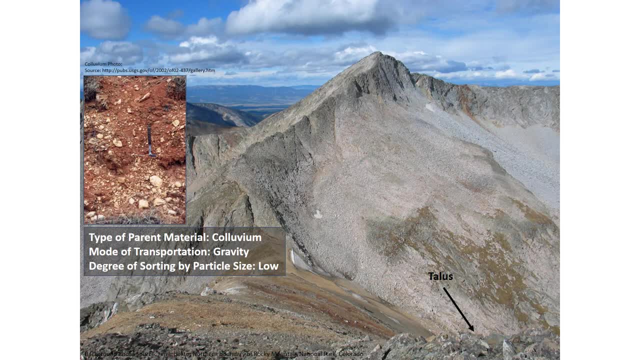 transported by gravity. Colluvium is made up of a heterogeneous mixture of boulders, rocks, pebbles and soil from upslope areas. thus the degree of particle sorting is low. Sand and rocks collected at the foot of a slope is talus. These are common in areas. 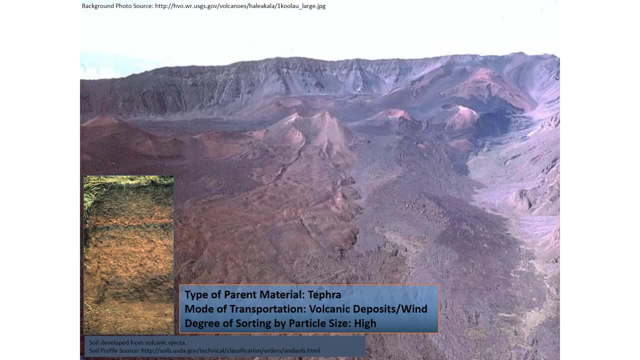 with mountains such as Arizona. The ash blown out of a volcano and deposited nearby or carried some distance by wind forms a chemically distinct, dark and lightweight parent material called pephra. The mode of transportation is wind. Wind is a good sorter of particles Larger. 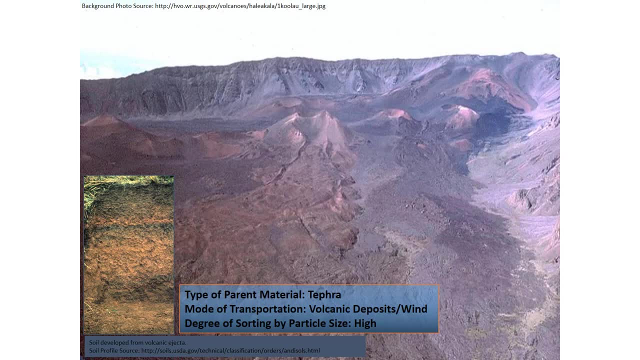 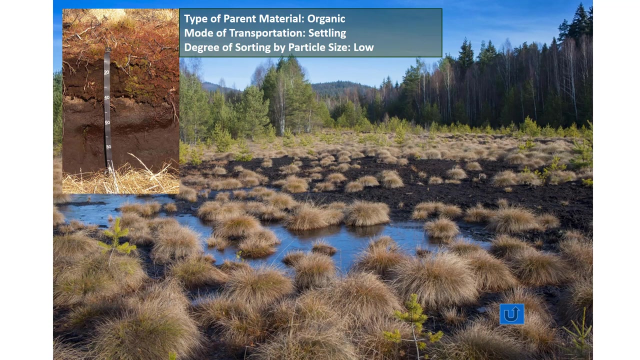 particles tend to bounce on the Earth's surface, while smaller particles are transported greater distances. The Pacific Northwest, Hawaii and Alaska are areas of the United States where such deposits are common. Organic soils containing 20% or more organic matter form underwater as aquatic plants die. Low oxygen conditions, underwater retard. 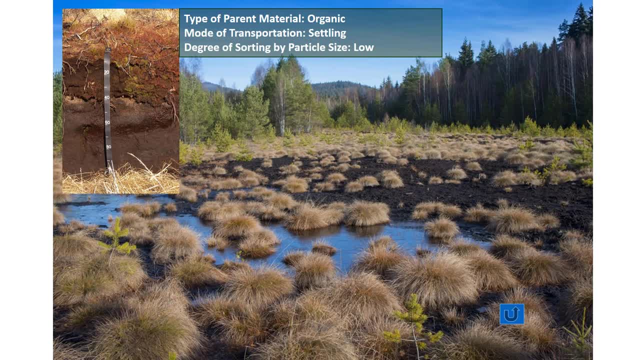 decay of these dead plants, so partially decayed remains, such as sand rocks, pebbles and stones, tend to pile up at the lake bottom. Organic soils are extensive in Minnesota, Wisconsin, Florida, Michigan and Alaska. When climate is extremely complex, we are 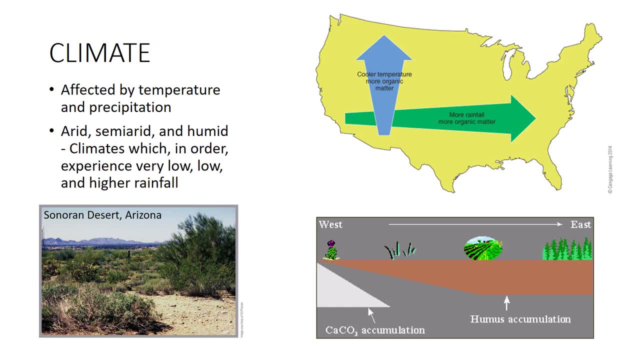 speaking here primarily of temperature and precipitation. Arid, semi-arid and humid refers to climates that experience very low, low and higher rainfall respectively. Climate first affects soils, causing physical and chemical weathering of rock. Temperature affects the speed of chemical reactions in the soil. 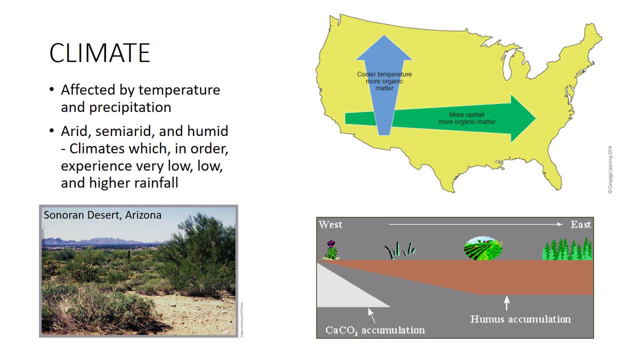 The higher the temperature, the faster a reaction. Chemical weathering in soils occurs mostly when the soil is warmer than 60 degrees Fahrenheit. Thus in cold areas, such as tundra, soils develop slowly. In warm areas, such as the tropics, soils develop more rapidly. Another 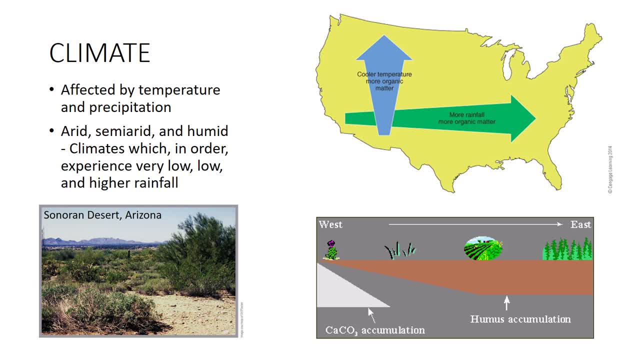 result of temperature is its effect on organic matter. Warmth promotes greater vegetation, so more organic matter is added to the soil. However, warm temperatures also speed the decay of soil. The soils of warm temperatures tend to be low in organic matter. In warm regions, warmth- 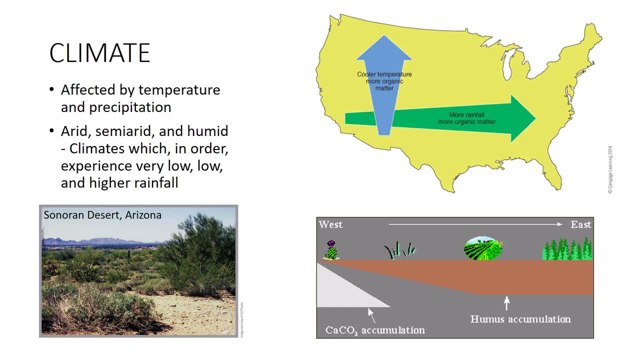 promotes dissolution of materials, so if climate is also humid, chemicals leach out of the soil more quickly. Warm climates also promote the weathering of clay minerals to forms that are less fertile. Soils of this piece of the Sonoran Desert near Phoenix are influenced by sparse vegetation. 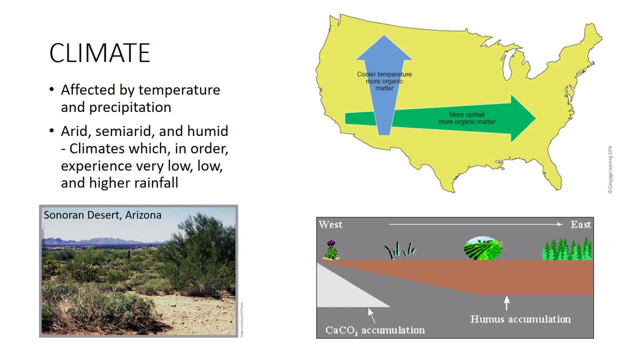 and arid climate. Desert soils tend to be enriched in salts that would leach out the soil in humid climates. In this diagram in the United States it shows that the average organic matter increases to the east and north because of higher rainfall or cooler temperatures. 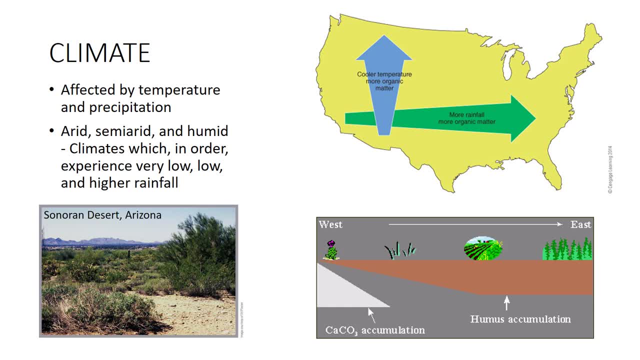 Other factors also affect organic matter, like vegetation, which alters these trends regionally. Another effect of climate is on soil pH. Calcium carbonate accumulates in the western US, increasing pH. Calcium carbonate accumulates in the western US, increasing pH. and humus accumulates in the eastern US, decreasing pH. 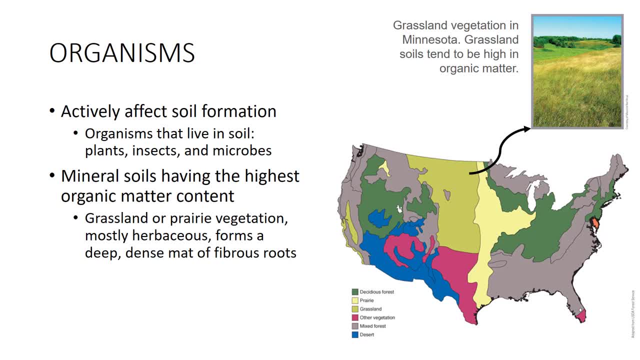 Organisms that live in soils, such as plants, insects and microbes, actively affect soil formation. The actual properties of a developing soil are influenced especially by the type of plants growing on it. The figure shows the parent vegetation of soils of the United States: Mineral soils. 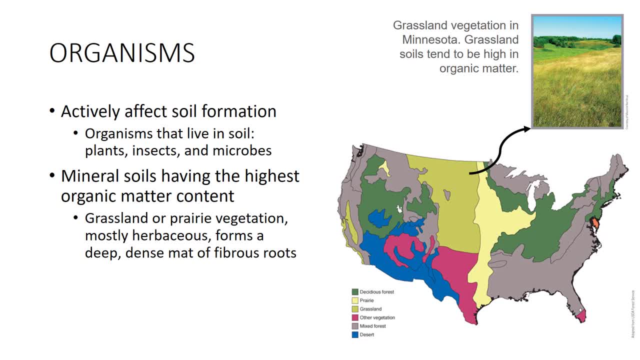 having the greatest organic matter content form. under grasslands or prairies, The soil contains a deep, dense mat of fibrous roots, many of which die each year and contribute large amounts of organic matter to the soil. Indeed, most of the biomass of a prairie develops. 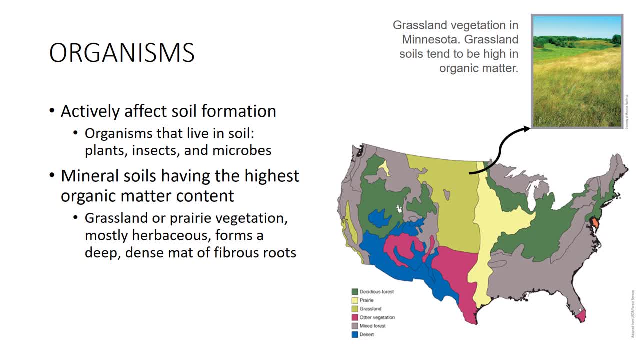 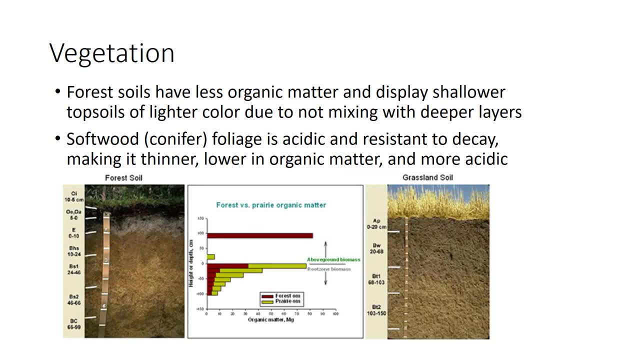 underground in the soil. This keeps their organic matter content high and the soil color dark. In a forest, much of the biomass grows above ground in the trees. When leaves fall or the trees die, they are not produced. The soil is covered in organic matter. This is what 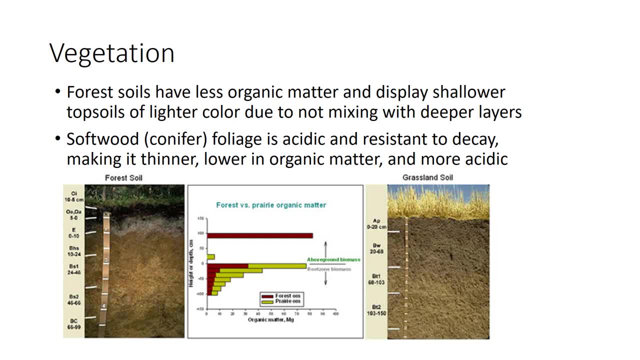 the soil is made of. The soil is made of organic matter. The soil is made of organic matter. The material falls to the soil, where it creates a surface layer of organic matter that does not mix with deeper layers. As a result, porous soils have less organic matter than prairie soils and 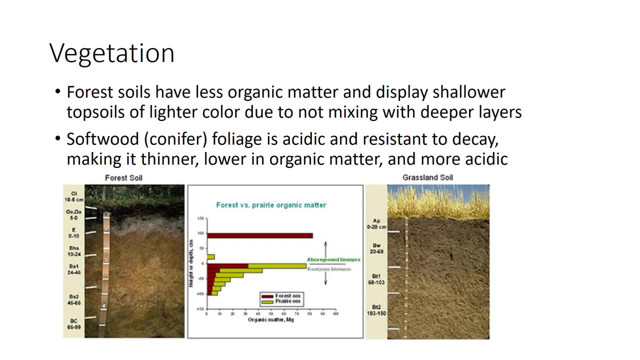 display shallower topsoils of lighter color. The type of trees also influences the soil. Compared to hardwoods, deciduous trees, softwood conifer foliage is acidic and resistant to decay. Therefore their soils tend to be thinner, lower in organic matter and more acidic. 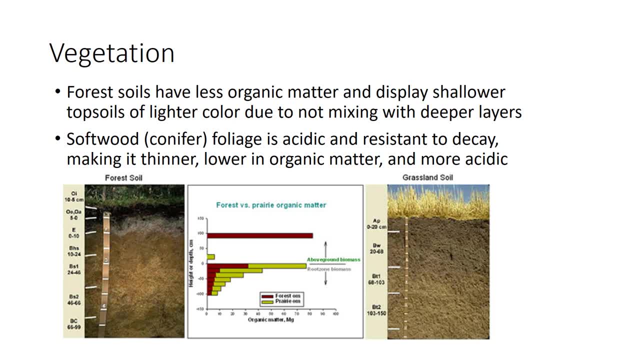 Deserts with very sparse vegetation have the least organic matter. Deep roots of deciduous trees extract ions from deep in the soil, leaving the surface horizon of deciduous forest soils enriched in ions. We tend to stress vegetation as the main living factor in soil. 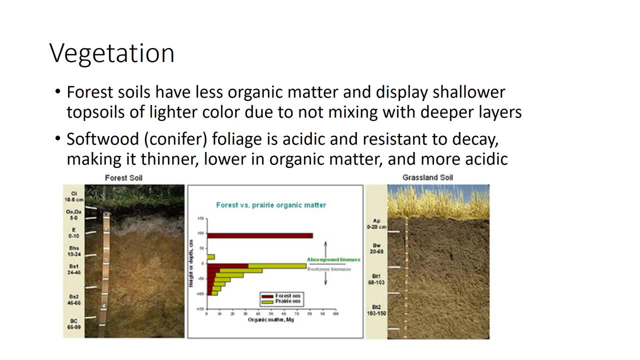 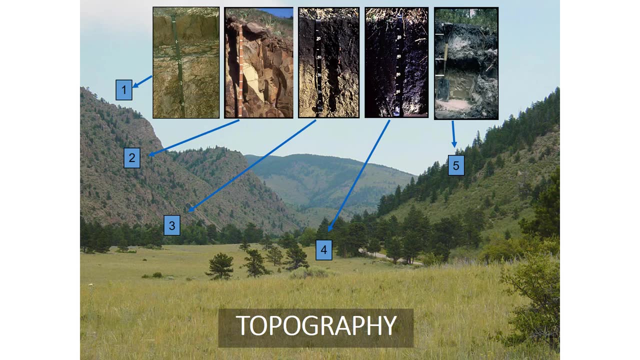 formation. but other life impacts soil as well, such as burrowing animals that mix the soil with the soil, Earthworms that create large, deep pores and speed organic matter decay or nitrogen-fixing bacteria. Topography or the soil's position in the landscape influences soil development mainly. 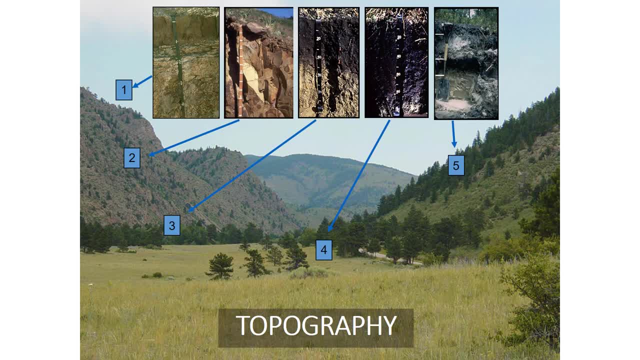 by affecting water movement and soil wetness. Major changes in soil type can occur over very small differences in elevation and distance. due to topography One, this soil developed on the hilltop, which is relatively flat. Therefore, the soil is relatively flat. The soil is relatively flat on the hilltop, which is relatively flat on the hilltop. 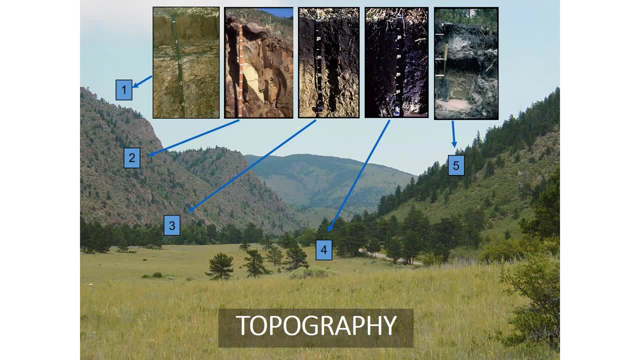 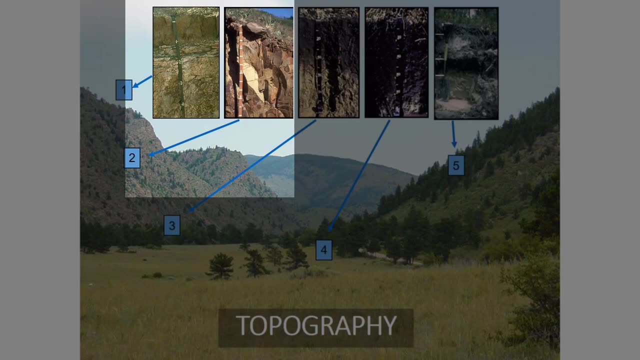 The soil is relatively deep and well-drained. It also received direct sun and is thus relatively dry, dominated by shrubs and, to a lesser extent, grasses. Two: this soil developed along the hill slope with a south-facing aspect. Soils are eroding due to. 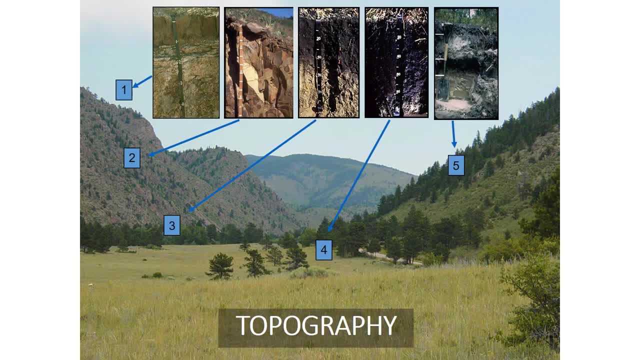 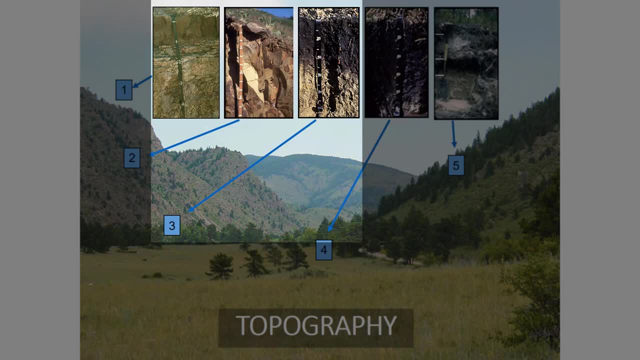 slope and thus there is relatively less soil development. This soil is dominated by grasses and, to a lesser extent, shrubs. Three: this soil developed along the toaster. This soil is relatively dry, dominated by shrubs and, to a lesser extent, grasses. 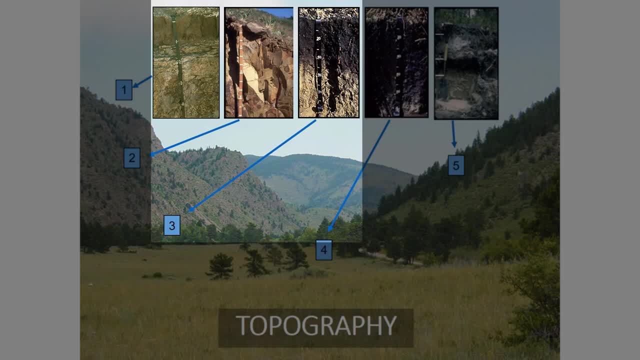 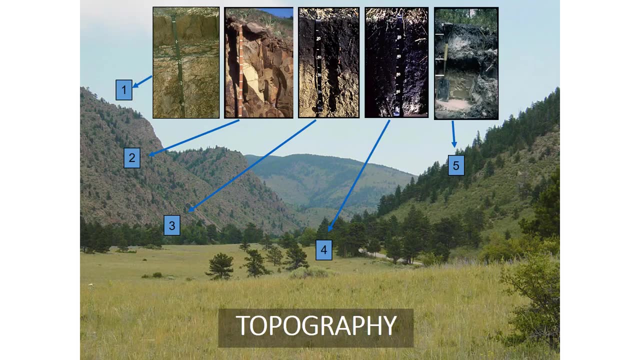 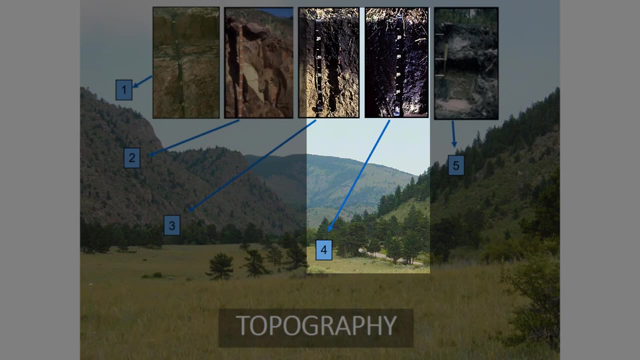 Soil is somewhat wet, as evident by the somewhat gray subsurface soil. This soil is dominated by grasses and some wetland plants. Four: this soil developed in the valley and is shaded by the northern slopes. Many soil materials, including mineral and organic matter, have eroded into this. 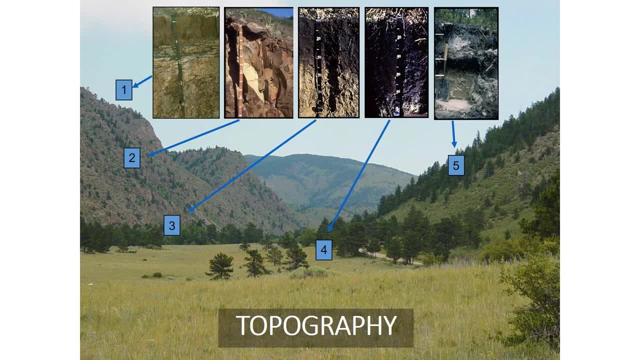 area. This area is low-lying and thus wet. A high water table is present, Thus the soil profile is slightly wet and is therefore affected by the south-facing aspect. The soil is somewhat wet as profile is relatively thick and dominated by wetland plants. 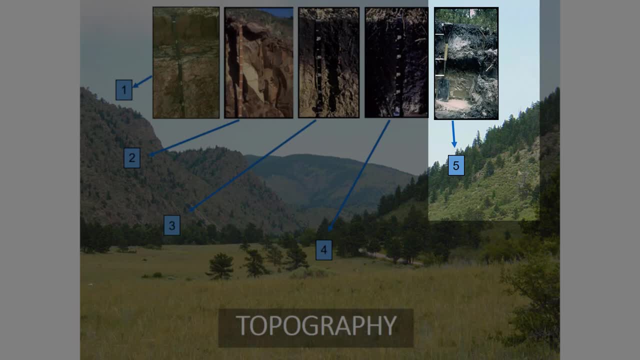 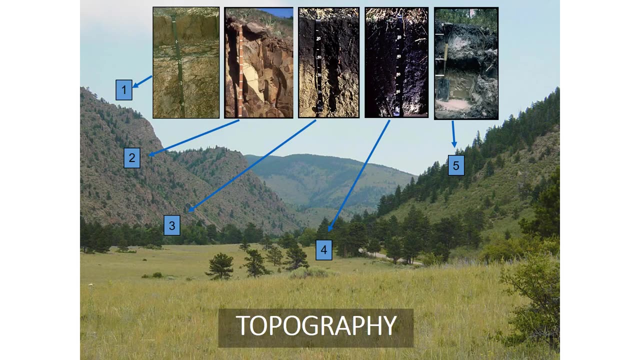 5. This soil developed on the north-facing aspect. thus they are cooler temperature-wise as compared to the south-facing soils. These soils support coniferous trees which deposit plant litter with an acidic pH. The litter accumulates on the surface and decomposes slowly. 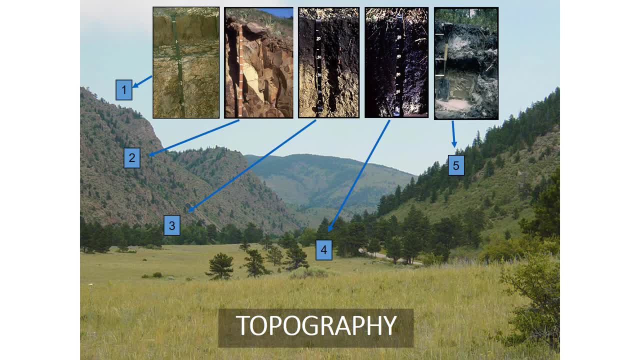 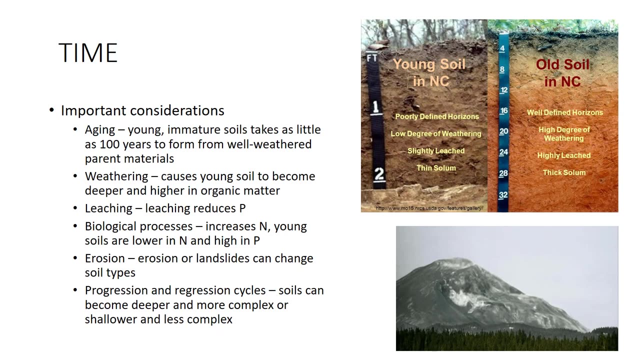 When it does decompose, it releases acid which causes the breakdown and movement of soil materials out of the white upper soil and redeposits materials in the lower, darker soil. Soils change over time, undergoing an aging process. Initially, a thin layer of soil appears on the parent material. 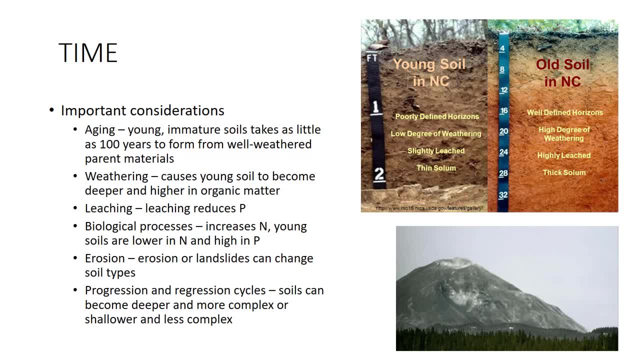 Such a young, immature soil takes as little as 100 years to form from well-weathered parent materials under warm, humid conditions. Under other conditions it may take hundreds of years. Weathering of the young soil continues and many generations of plants live and die. so the young soil becomes deeper. 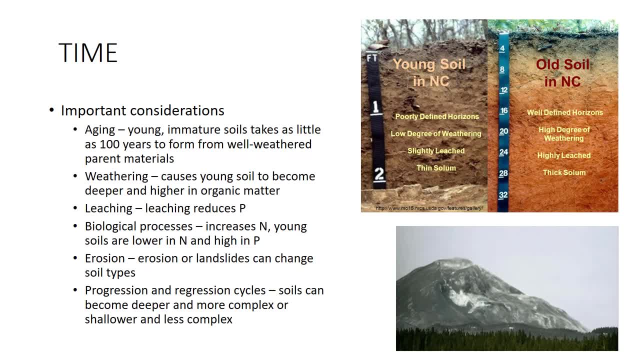 and higher in organic matter. If there is enough rainfall, leaching begins to carry some material deeper into the soil. As soils age, biological processes tend to increase the nitrogen content, while leaching tends to reduce phosphorus. Thus young soils tend to be low in nitrogen but high in phosphorus, while older soils 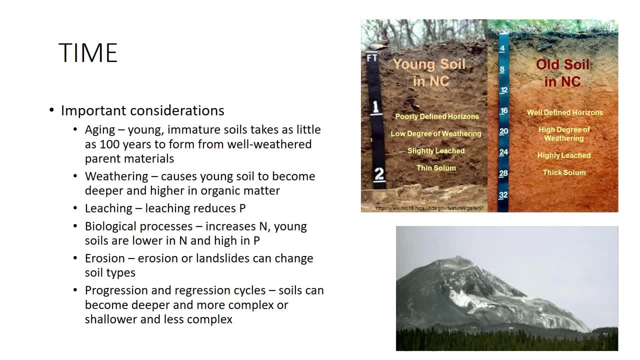 are the opposite. Mature soils are generally productive, But as soil continues to age, it becomes less and less. Soil changes over time. They become more severely weathered, more highly leached and often less productive In general. as soil ages, it becomes deeper, develops distinct layers and becomes more. 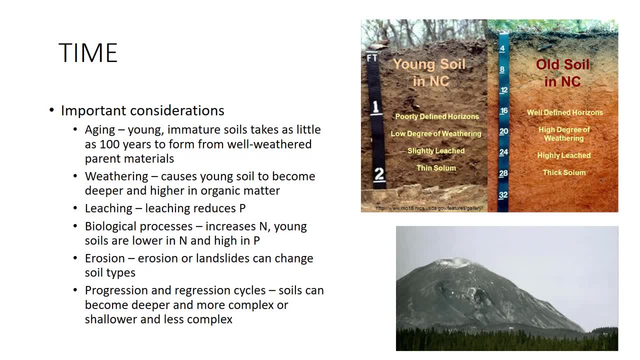 acidic and leached. Time zero for a soil usually begins when some dramatic event such as landslides, glaciers or piling a mining spoil, changes everything and resets the clock. Such events can happen at any time. Soils can erode away, be buried or even become the parent material. 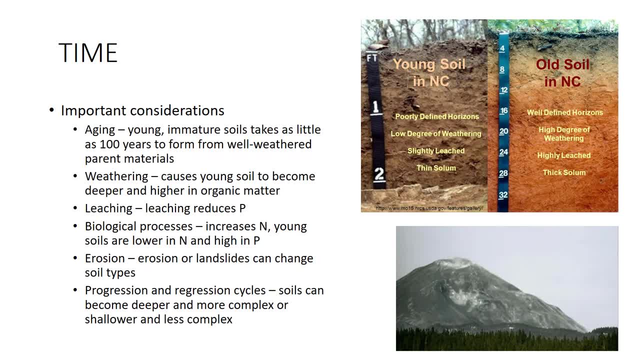 Soil can be buried or even become the parent material. Soil can be buried or even become the parent material. Soil can be buried or even become the parent material for a new soil. If soil factors change the direction of soil, development can be deflected into a new path. 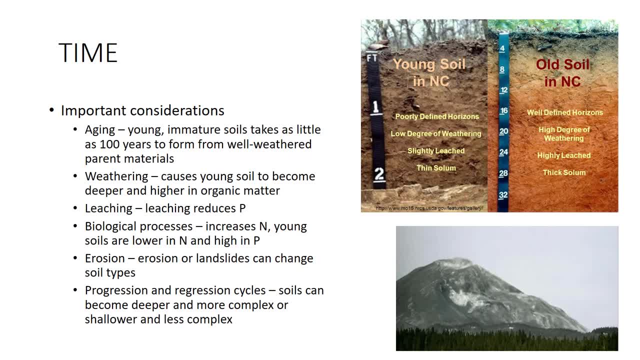 For instance, if a forest invades prairie, the soil embarks on a new path towards a forest-type soil. We tend to think of soil development as progressive, that is, soil becomes deeper and more complex, with more and better-defined layers. 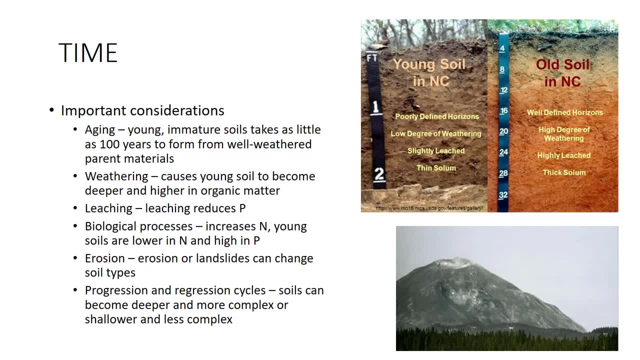 But if the combination of soil-forming factors changes, soil can also regress, becoming shallower and less complex. Very old soils may have undergone repeated cycles of progression and regression. Humans may be considered just another living entity that modifies soil, but their action 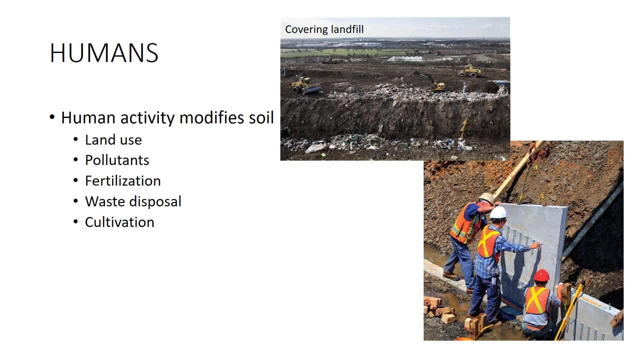 can be so rapid, dramatic and different from other life that they may be considered a separate six-soil formation factor. Very few soils have been unaffected by human activities. Effects may be as subtle as the deposition of air pollutants distant from any human habitation. 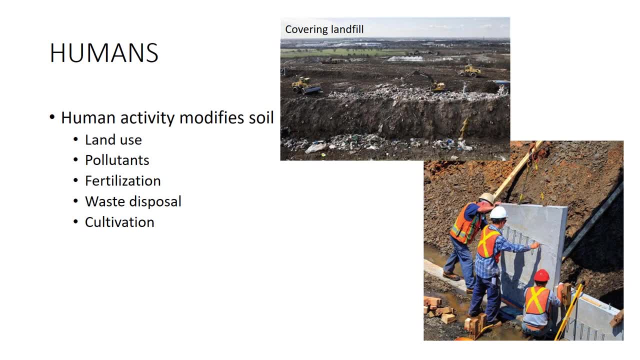 to as massive as earthworms. The earth moving during road construction: The latter resets the time clock for this new soil material to zero, and the earth moved by the machinery is the parent material for this new soil. Much of what people do to grow plants alters the soil, like cultivation or fertilization. 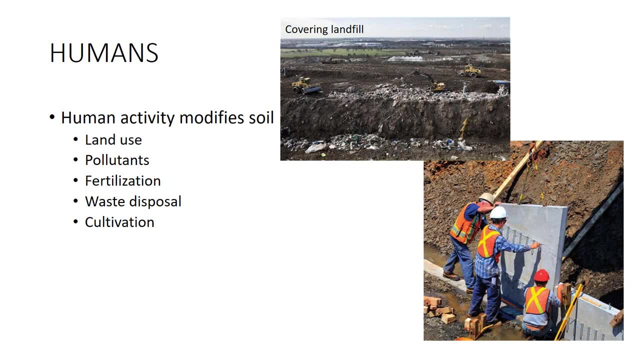 Humans also enrich soils around them in phosphorus by fertilization and disposal of garbage. This effect is distinctive enough that archaeologists use phosphorus enrichment as evidence of early human habitation. Our system of soil classification also recognizes such enrichment in some soils. Soils change over time in response to their environment, represented by the soil-forming. 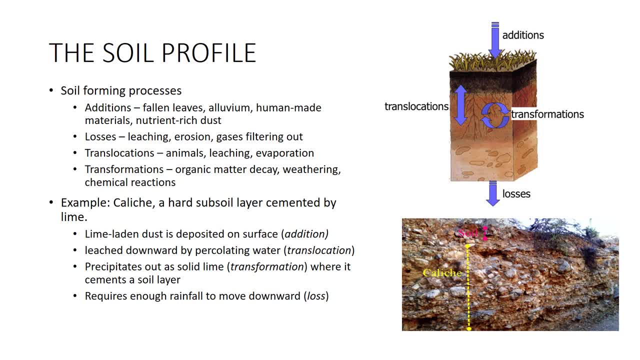 factors. Soil scientists have classified the causes of those changes into four soil-forming processes. Additions: Materials may be added to the soil. Some examples are fallen leaves, alluvium and human-made materials such as air pollutants and compost. Deposition of nutrient-rich dust is a major contributor to the fertility of many soils. 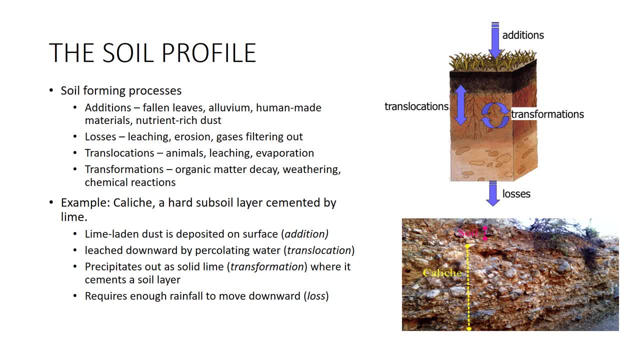 Losses: Materials may be lost from the soil as a result of such mechanisms as deep leaching, erosion from the surface or gases filtering out of the soil. Translocations: Materials may be moved within the soil by leaching deeper into the soil. 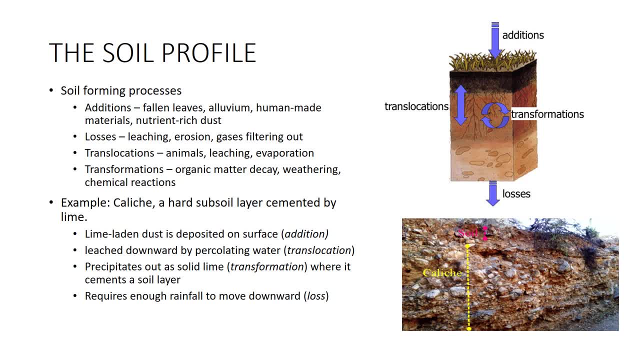 by being carried upward with evaporating water, by being moved by animals such as ants or earthworms, Or by other actions. Soil optimization: that moves soil material around. Transformations: Materials may be altered in the soil, For example organic matter, decay, weathering of minerals to smaller particles or chemical reactions. 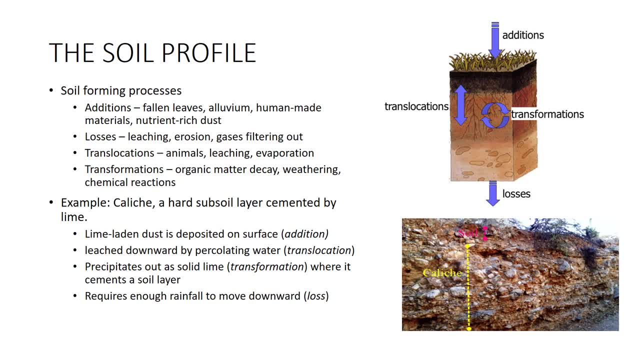 For example, some soils contain caliche, a hard subsoil layer cemented by lime. Its formation has been explained this way: Over long periods of time, lime-laden dust is deposited on the soil surface Addition. It is leached downward by percolating water Translocation And precipitates. 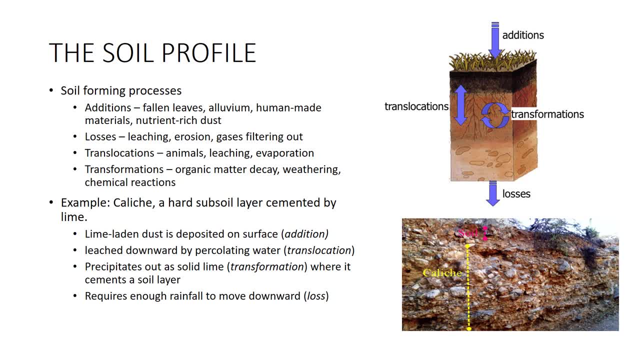 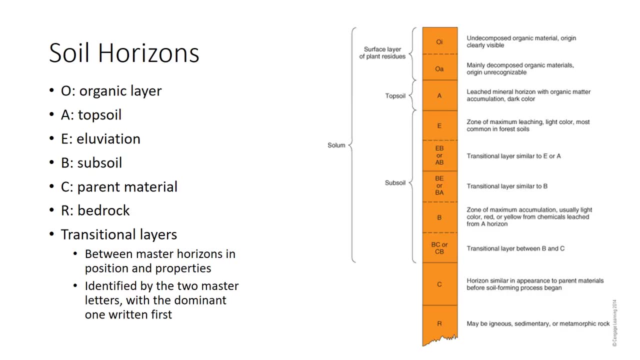 out as solid lime at some depth Transformation, Where it cements a soil layer. This process requires the correct amount of rainfall: enough to translocate the lime downward, but not so much as to move it out of the soil altogether. Loss: Each of these processes occurs. 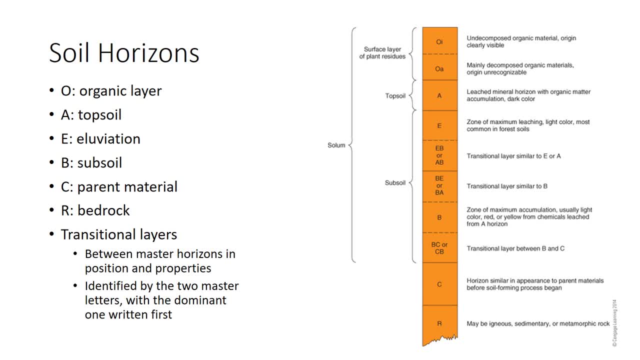 differently at different depths. For instance, organic matter tends to be added at or near the surface, not deep in the soil. Some material moves from high in the soil to be deposited lower. As a consequence, different changes occur at different depths and horizontal 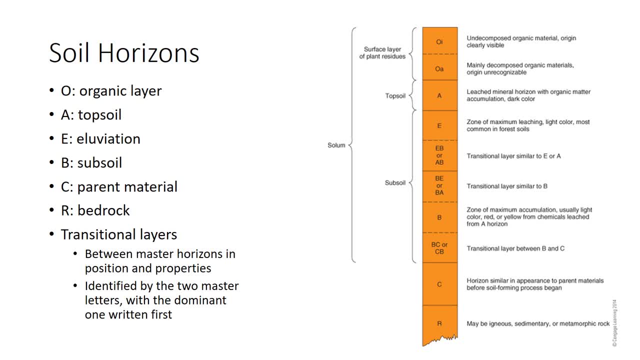 layers develop as the soil ages. These layers are known as soil horizons, visible wherever the earth is dug deep enough to expose them. The soil profile is a vertical section through the soil, extending into unweathered parent material and exposing all the horizons. 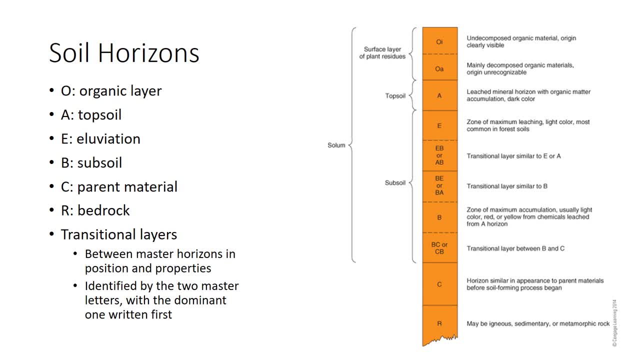 Each horizon is a vertical section through the soil extending into unweathered parent material and exposing all the horizons. Each horizon in the profile differs in some visible, physical or chemical way from other horizons. The O horizon is an organic layer made of wholly or partially. 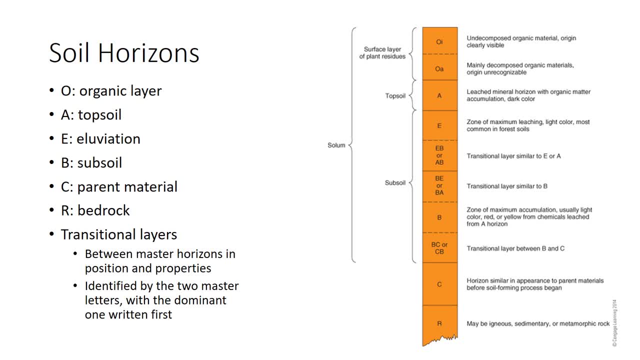 decayed plant and animal debris. The? A horizon, called topsoil by most growers, is the surface mineral layer where organic matter accumulates. It is darker than the horizons below. Over time, this layer loses clay, iron and other materials in downward moving water, A loss called alluviation. 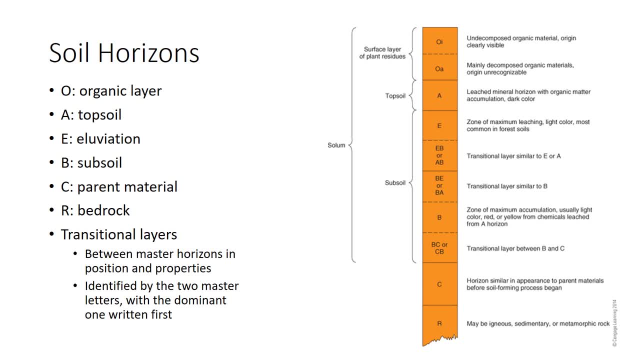 The E horizon, the zone of greatest alluviation, is very depleted in clay, chemicals and organic matter. Because chemicals that color soil have been leached out, the E layer is very light-colored. Many soils have no E horizon. It is most likely to occur under forest vegetation and sandy soils. 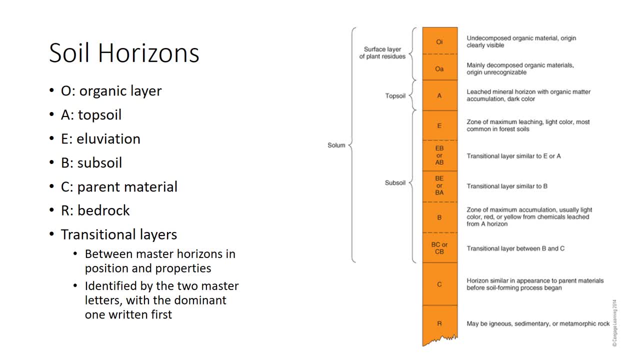 in high rainfall areas. The B horizon, or subsoil, is often called the zone of accumulation, where chemicals leached out of the A and E horizons accumulate. The C horizon lacks the properties of the A and B horizons: It is the soil layer. 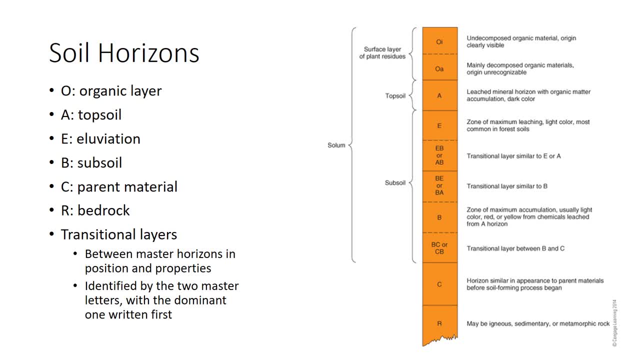 little touched by soil-forming processes and is usually the parent material of the soil. The R horizon is underlying hard bedrock such as limestone, sandstone or granite. It may be cracked and fractured, allowing some root penetration. The R is identified only if 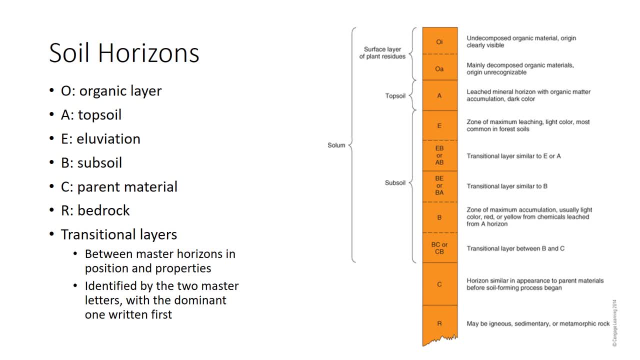 it is near enough the surface to intrude into the soil. When soils age, they may develop more horizons than the basic master horizons. These transitional layers are identified by the two master letters, with the dominant one written first. Thus, an AB layer lies between the A and B horizons and resembles both, but is more like the A. 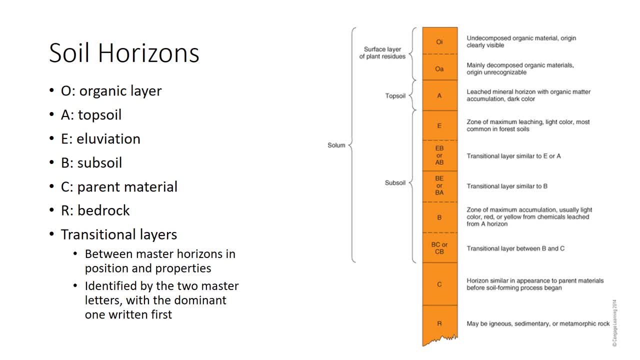 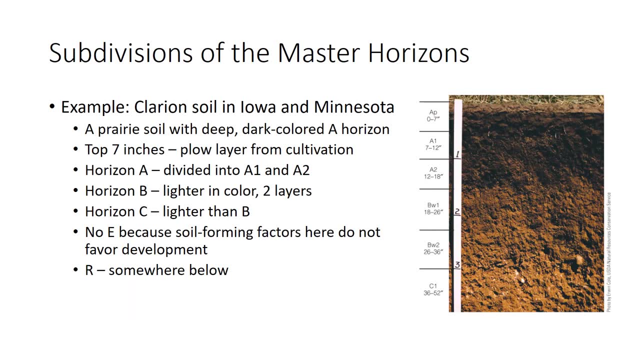 than the B A soil layer can be further identified by a lowercase letter suffix that tells some trait of the layer. Now, for an example, This photo shows the top 42 inches of the clarion soil found in Iowa and Minnesota. Clarion is a prairie soil with a deep, dark-colored A horizon. The top 7 inches are a plow layer. 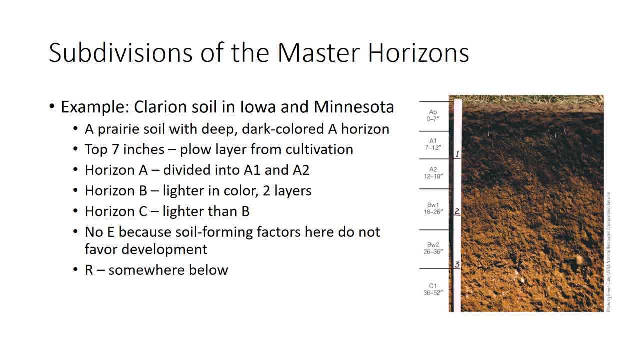 from cultivation, hence labeled AP. The thick A horizon extends below the plow layer and is divided into an A1 and an A2.. The differences between them are not readily visible in this photo. This makes the total horizon 18 inches deep.